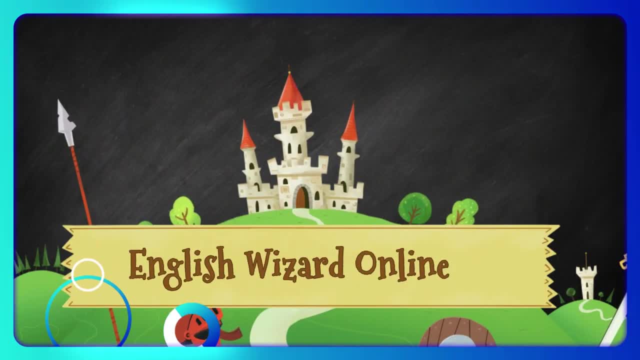 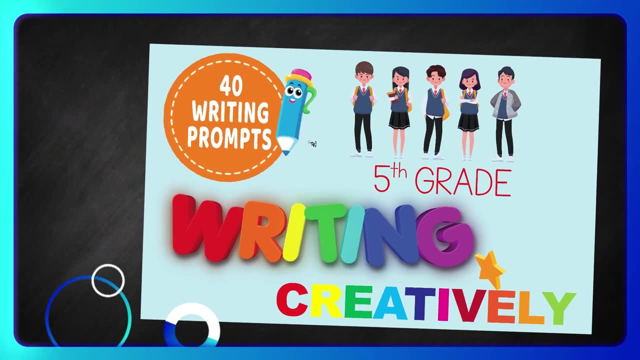 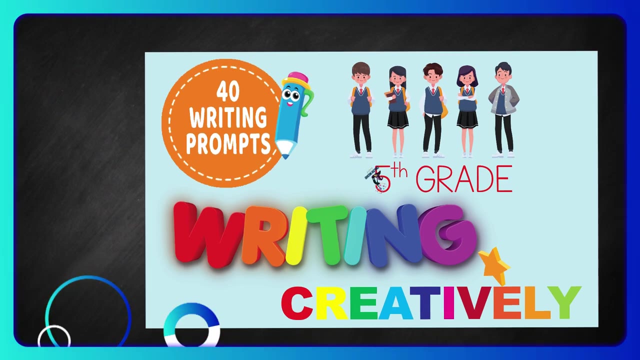 Creative writing develops creative thoughts, using imaginations, suggest alternatives, broaden thought process and problem-solving abilities. It also allows the child to show their opinions and develop their voice and improves their logical skills. Use these creative writing prompts for 5th grade. 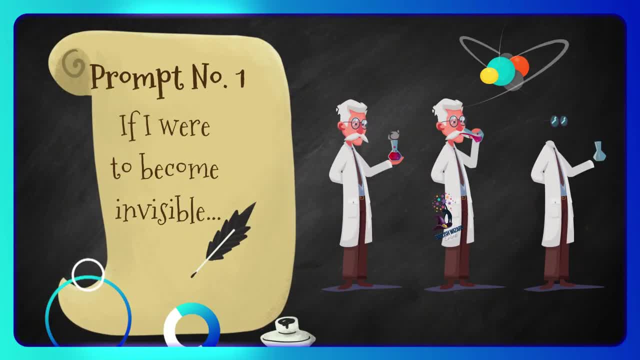 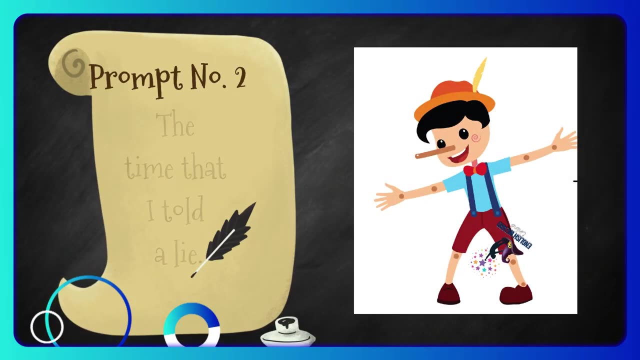 Writing prompt number 1. If I were to become invisible? Invisibility is indeed a superpower, and so being invisible is a good thing. What do you think would happen if you were to become invisible? Writing prompt number 2.. The time that I told a lie. 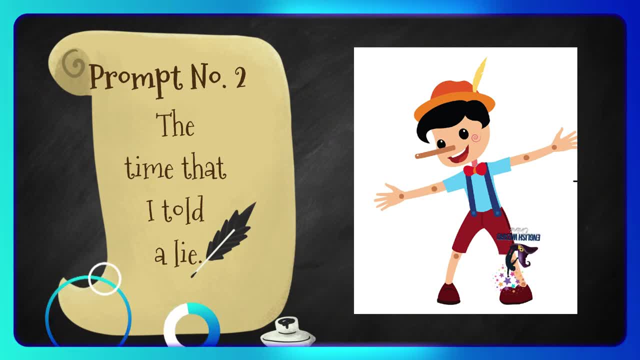 A lie is a mutual thought that your brain is telling you to do at a certain time. But lies always become bigger and can become something. Write about the time that you told a lie. Writing prompt number 2.. If I were to become invisible? 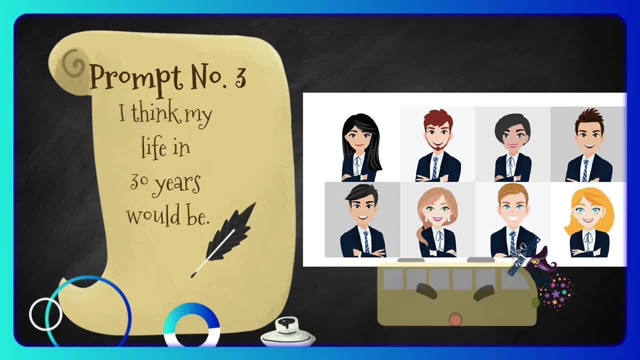 Writing prompt number 3.. I think my life in 30 years would be. It is hard to think about the future when one has not experienced much of life. There are so many paths that you could take. Imagine how you think your life in 30 years would be. 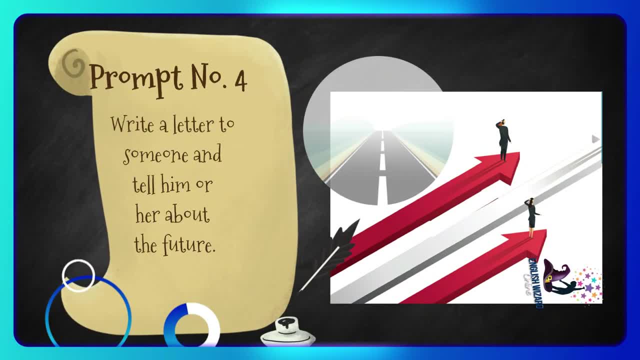 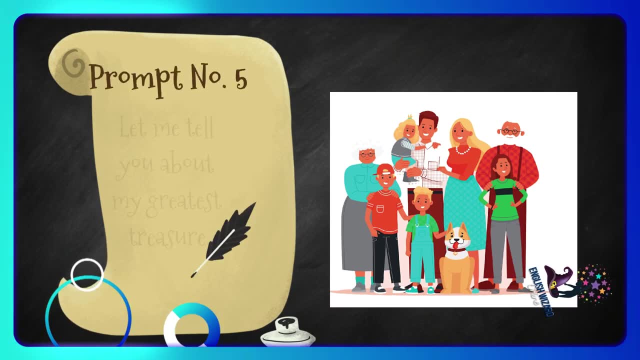 Writing prompt number 4.. Write a letter to someone and tell him or her about the future. Writing prompt number 5.. Let me tell you about my great-grandfather. Writing prompt number 6.. Let me tell you about my greatest treasure. 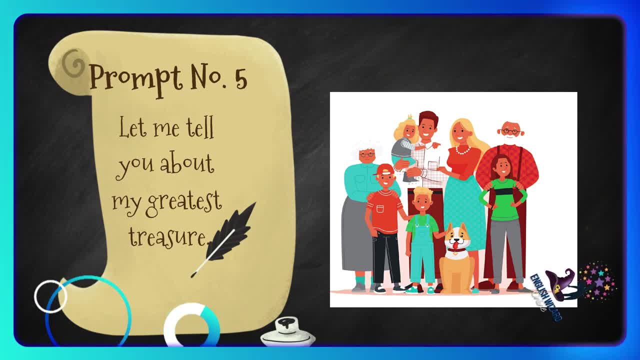 The English word treasure comes from the old French tresor, both meaning something of great worth. Treasure is defined as to find value in a person or thing. If you treasure something that you have, you keep it or care for it carefully because you think it is very special. 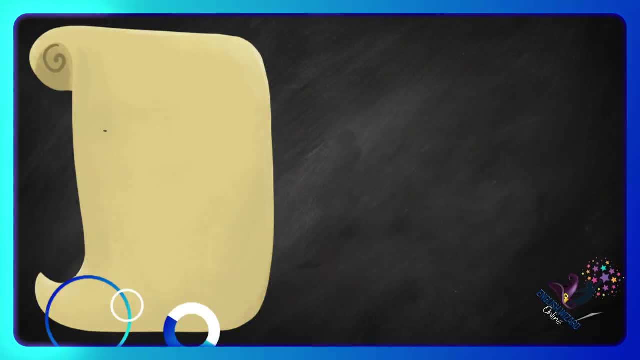 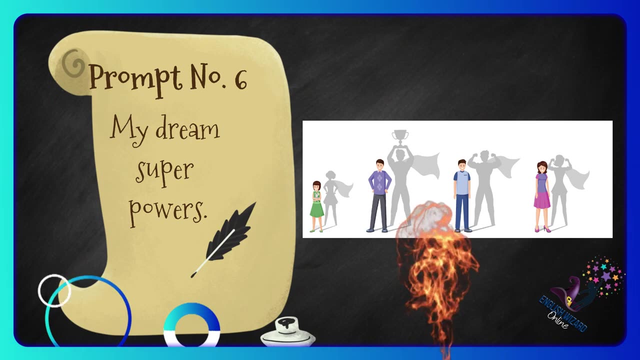 Write about your greatest treasure. Writing prompt number 6.. My dream superpowers. Writing prompt number 6.. My dream superpowers. Superpowers represent feelings of being confident or empowered about yourself, Your abilities more than usual, A display of superior strength or skill so incredible that it defies belief or expectations. 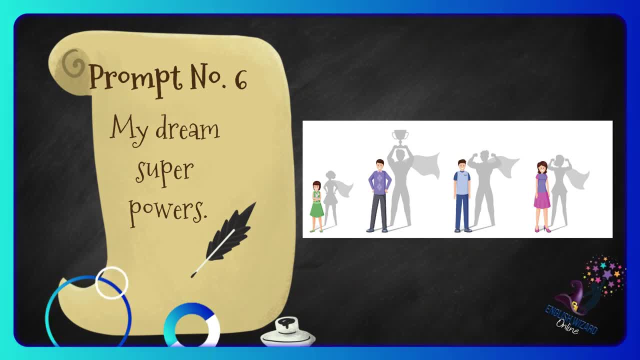 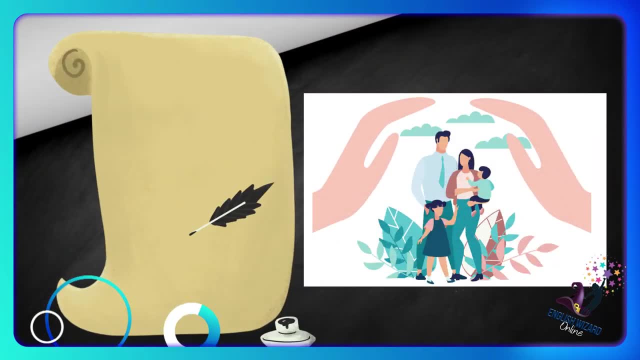 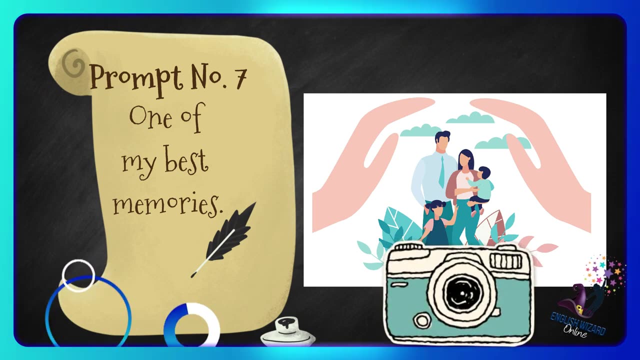 Surprising yourself with how powerful, effective or unstoppable you are. Write about your dream superpowers. Writing prompt number 7.. One of my best memories. Memories are one of the most crucial things which we can cherish throughout the life. They build up personality as knowledge and power. 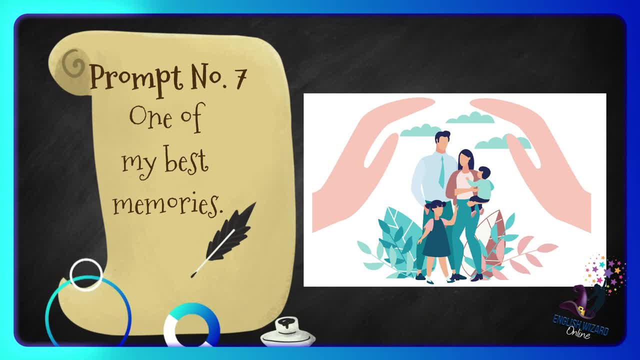 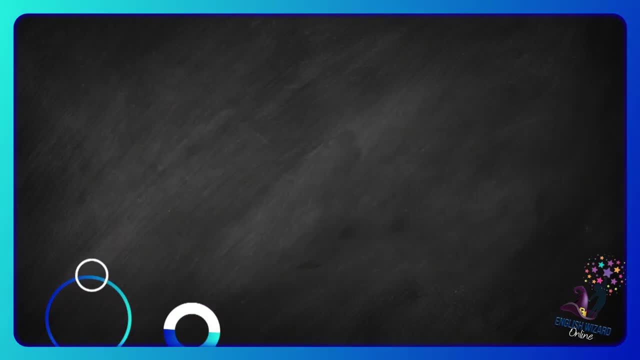 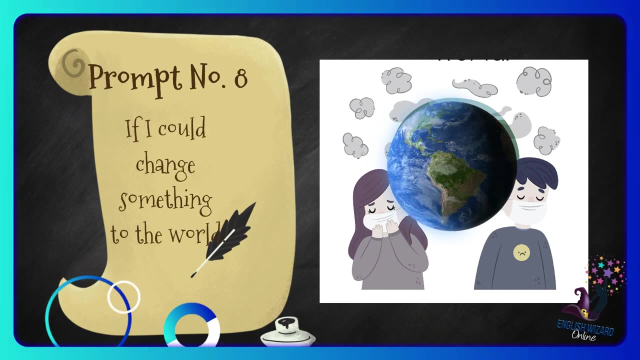 And previous experiences are stored there. Memories can be both good and bad. There are memories either from long ago or from recent past. Writing prompt number 8.. If I could change something to the world. In today's society there is so much that we might want to change about the world, but just don't have the means or power to do so. 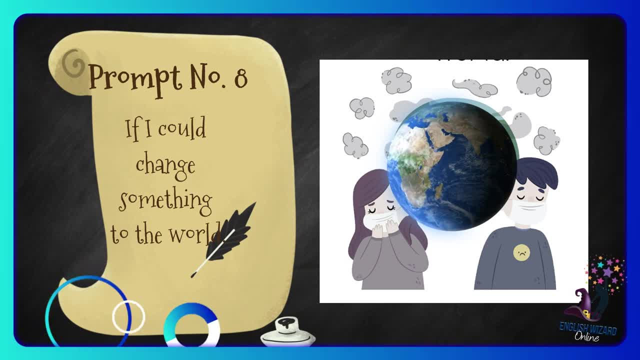 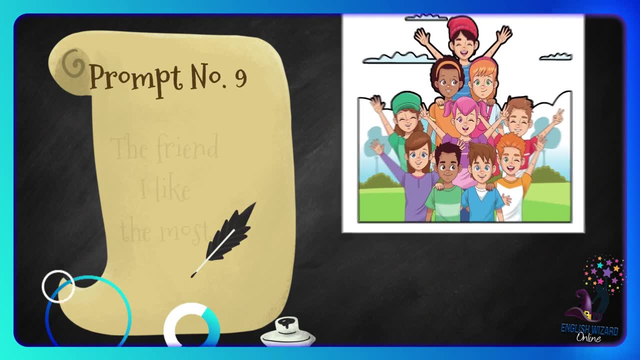 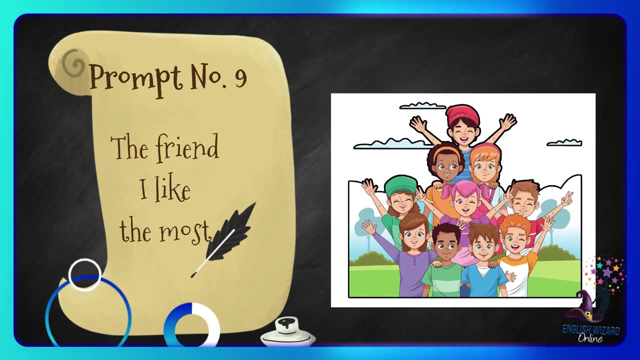 But what if you could change something to the world? What would it be? Write about it? Writing prompt number 9.. The friend I like the most. We come across lots of people every day. We interact with them. Some of them are relatives, but many belong to friend circle. 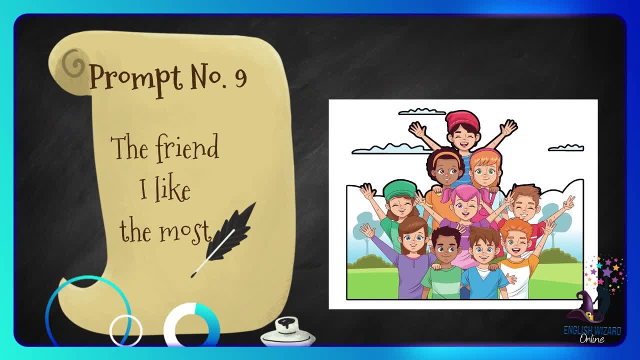 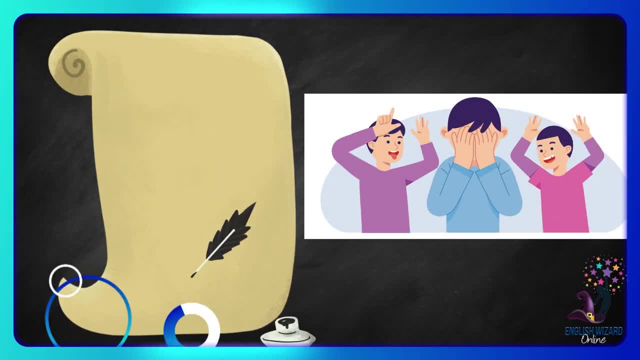 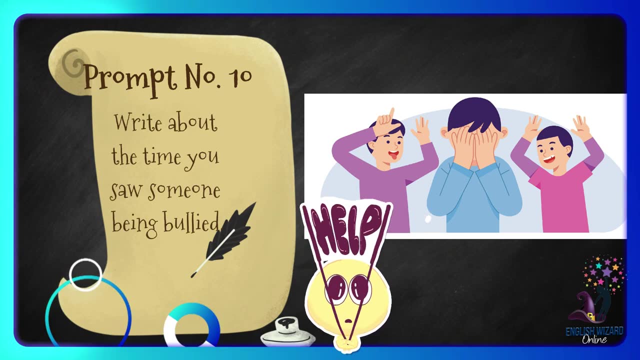 While some of them drift away, others remain close. Write about the friend that you like the most, Writing prompt number 10.. Write about the time you saw someone being bullied. Bullying is an intentional behavior that hurts, harms or humiliates a student. 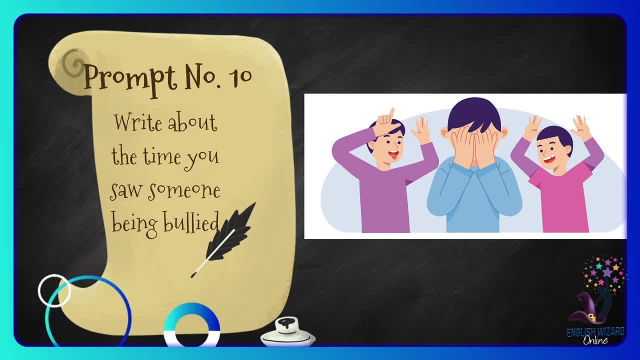 either physically or emotionally and can happen while at school, in the community or online. Those bullying often have more social or physical power, while those targeted have difficulty stopping the behavior. The behavior is typically repeated, though it can be a one-time incident. 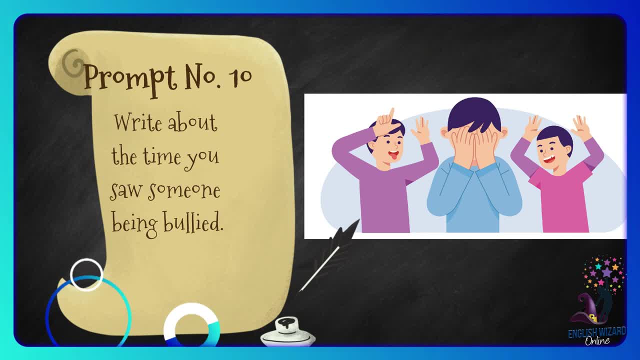 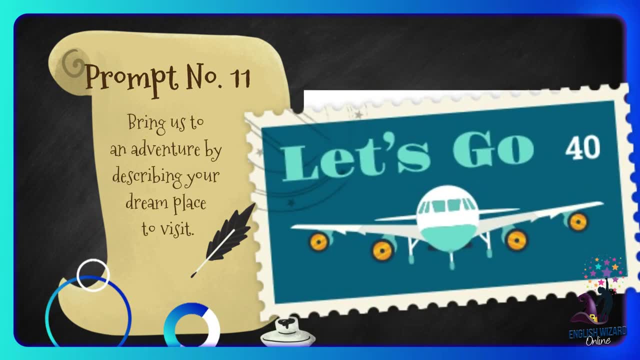 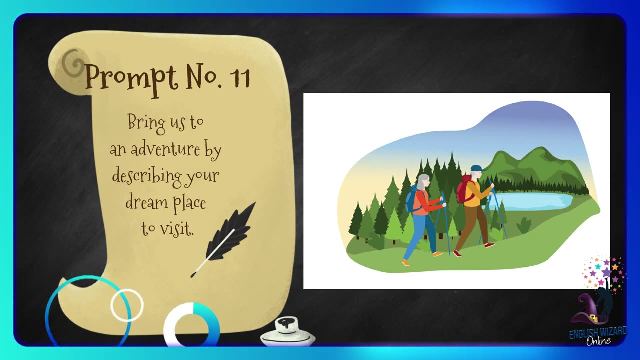 Write about the time that you saw someone being bullied. Writing Prompt Number 11. Bring us to an adventure by describing your dream place to visit. Adventure is an exciting, bold and risky activity, full of potential and dare, which gives an unusual experience to the people who try adventurous activities. 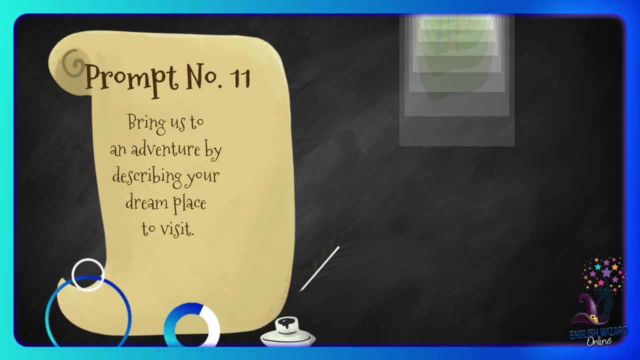 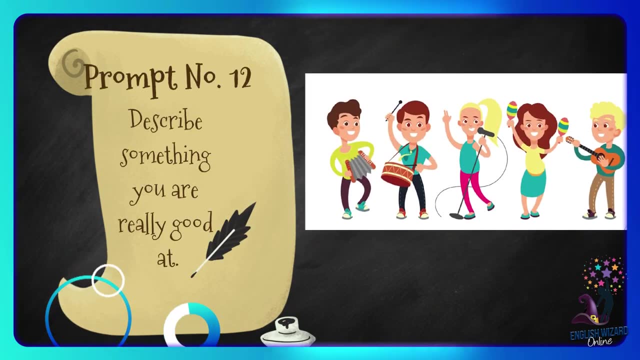 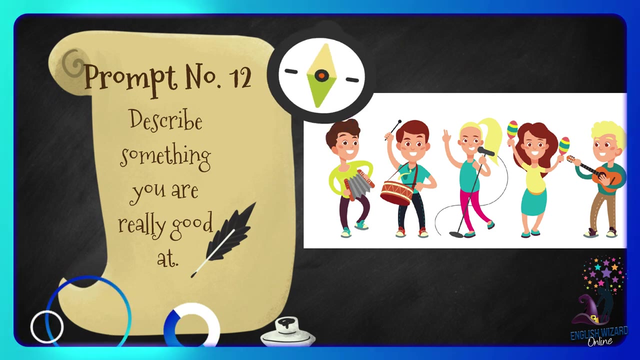 Write about an adventure by describing your dream place to visit. Writing Prompt Number 12: Describe something you are really good at. Do you have a hidden talent or skill? Talent is often thought of as a skill. Talent is often thought of as the kind of ability that comes without training and something that you're born with. 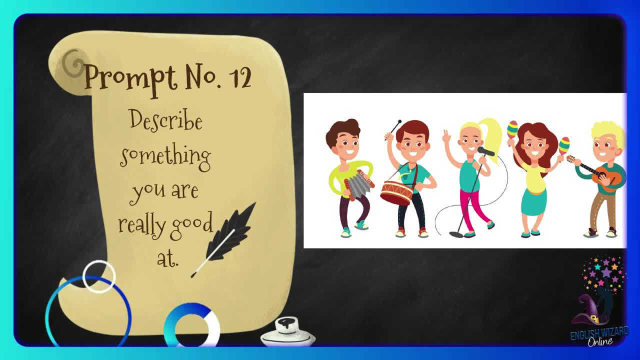 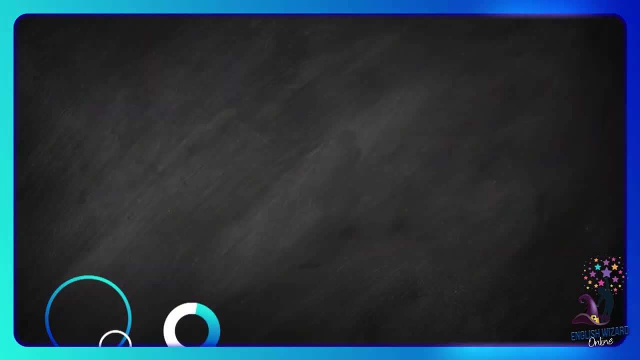 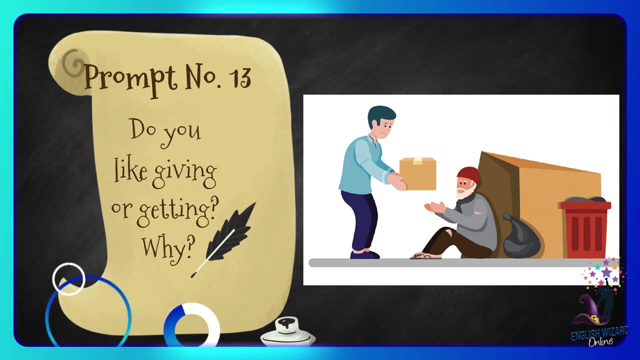 Skill, on the other hand, is an ability acquired and developed through practice. Write about something you are really good at. It might be a talent or a skill. Writing Prompt Number 13: Do you like giving or getting? Why, Between opening gifts from someone or giving gifts to someone, what would you prefer? 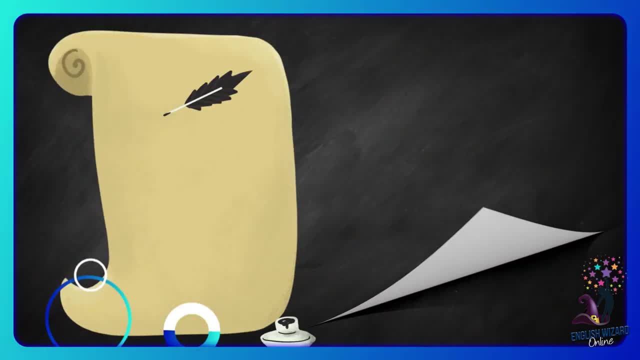 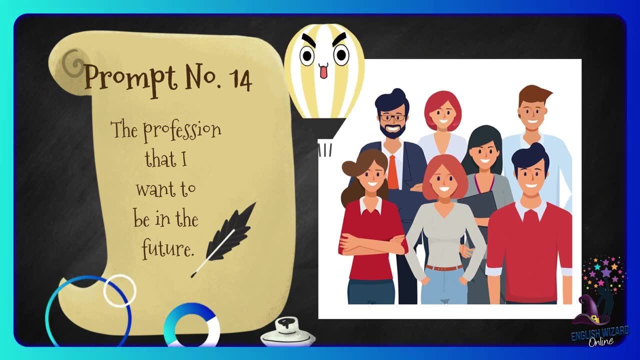 Write about it. Writing Prompt Number 14: The profession that I want to be in the future. Every person dreams of becoming someone in the future. It might be an engineer, a teacher, a doctor, a lawyer, a policeman or others. 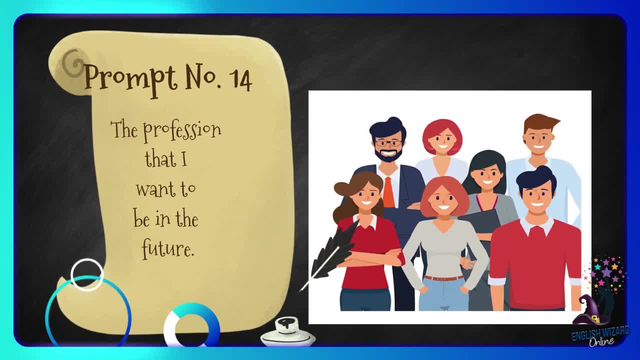 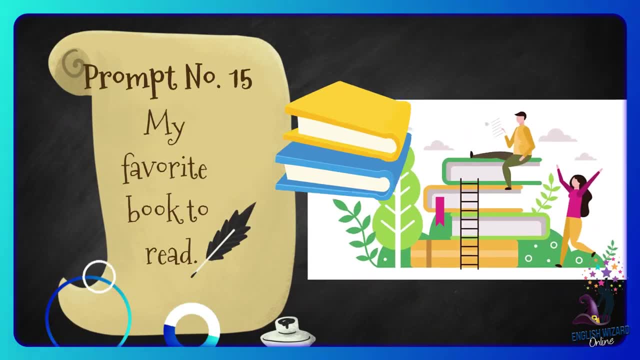 What profession do you want to be in the future? Write about it. Writing Prompt Number 15: My favorite book to read. Reading is important because it develops our thoughts, gives us energy and gives us the ability to think. It provides endless knowledge and lessons while keeping our minds active. 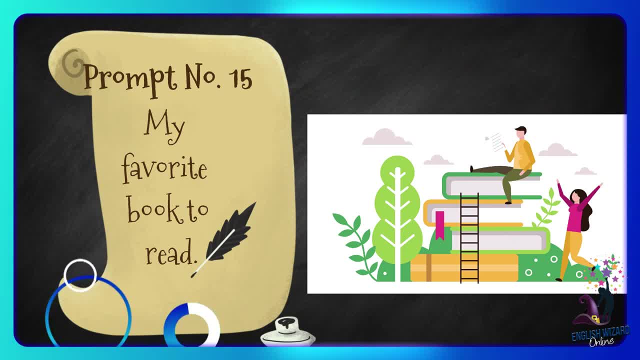 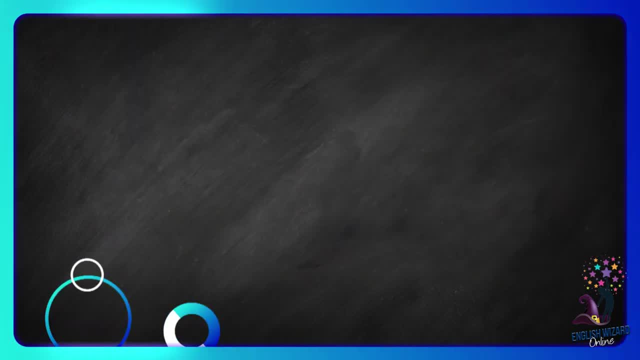 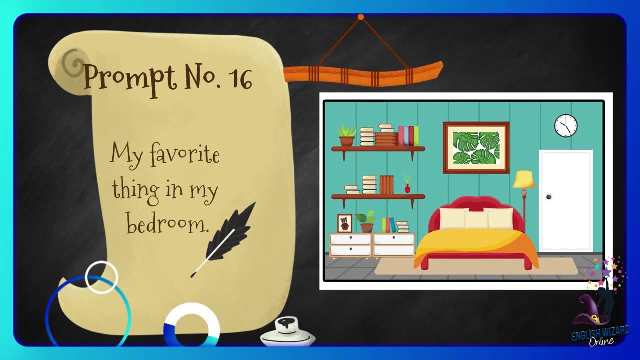 Books can hold and keep all kinds of information, stories, thoughts and feelings, unlike anything else in this world. Write about your favorite book to read. Writing Prompt Number 16: My favorite thing in my bedroom- Falling in love with a place fills up your heart with a sense of being home. 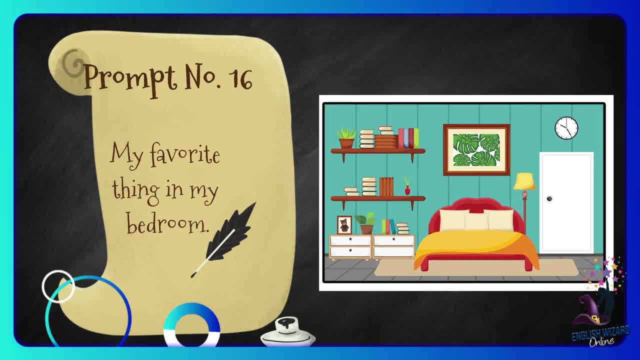 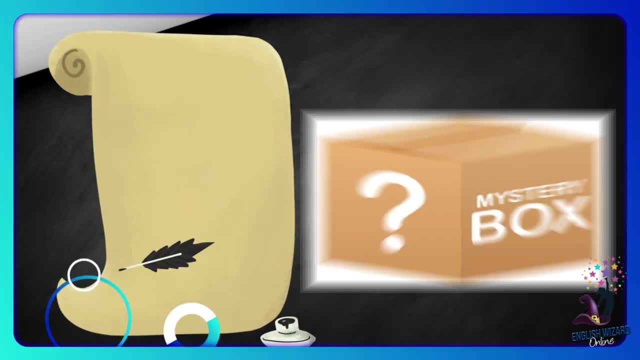 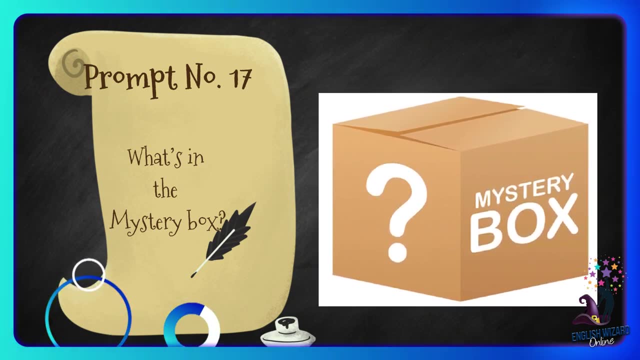 Sometimes we also get emotionally attached with our stuff in the room. Writing Prompt Number 17: What's in the mystery box? A mystery box is a surprise box that is often offered in a specific theme or brand. The content of the box will remain a surprise until delivery. 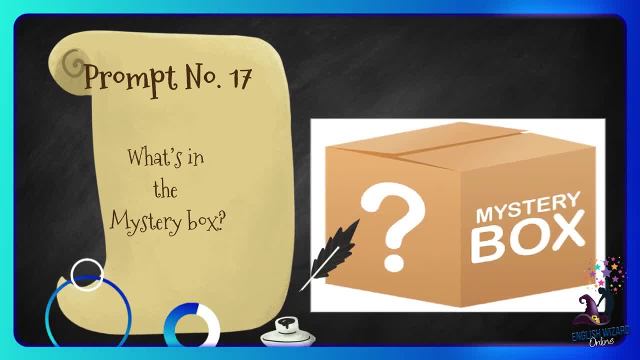 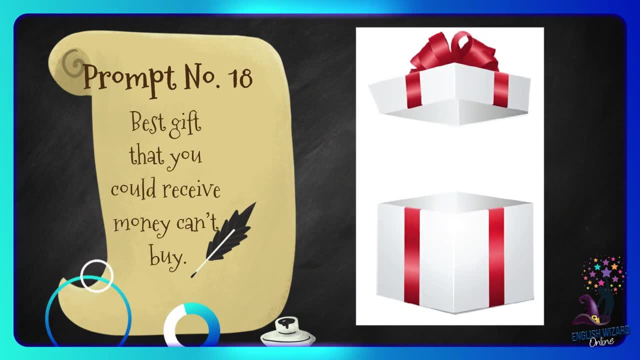 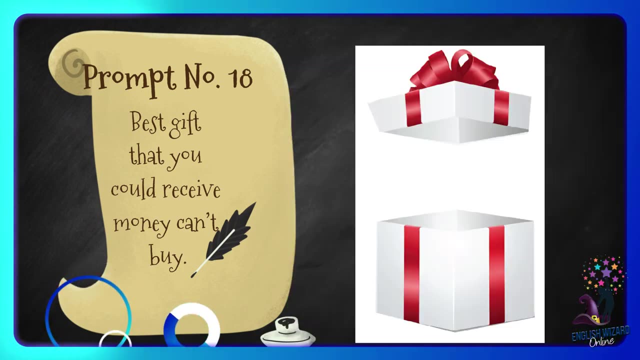 Use your imagination and pretend that you get a mystery box. write what's in it. Writing Prompt Number 18: Best gift for your family: What best gift that you could receive? money can't buy. Not everything great costs money. Sadly, now is also a time when we get so caught up in the materialistic things and objects. 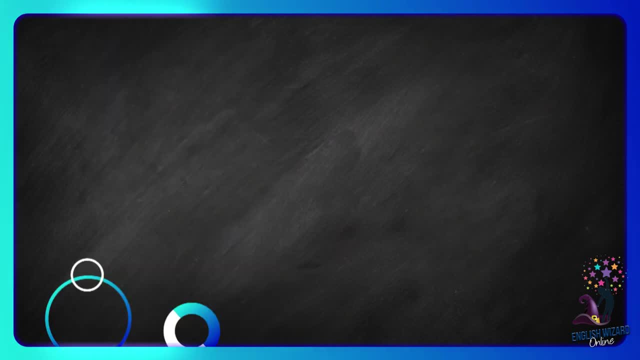 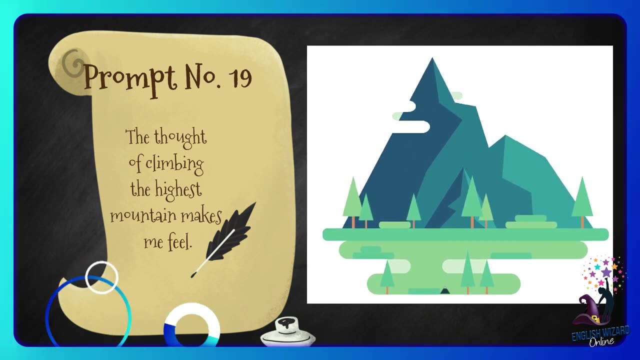 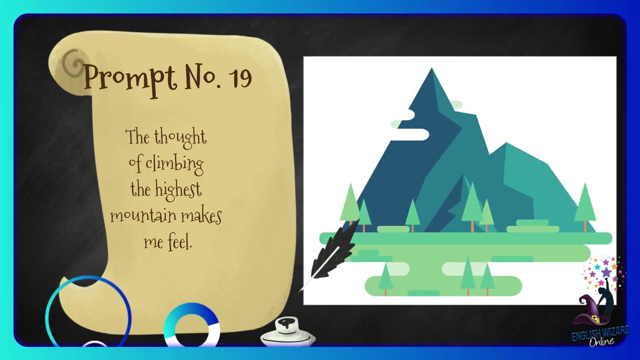 What best gift that you could receive? money can't buy Writing Prompt Number 19. The thought of climbing the highest mountain makes me feel Many dream of summiting the world's tallest peak. How does climbing the highest mountain make you feel? Write about it. 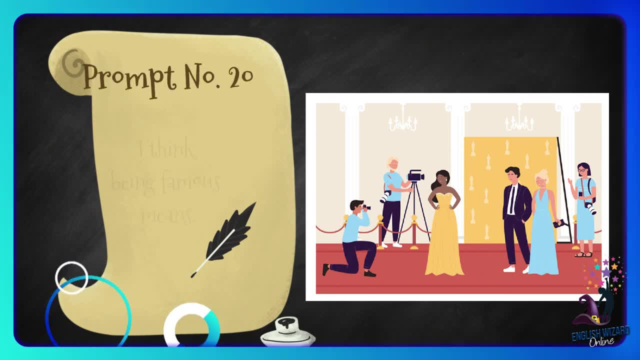 Writing Prompt Number 20. I think being famous means Some people become famous because of their natural talents. These people might be famous for singing, acting or hitting a baseball. Your natural beauty might even lead you to become a famous supermodel one day. 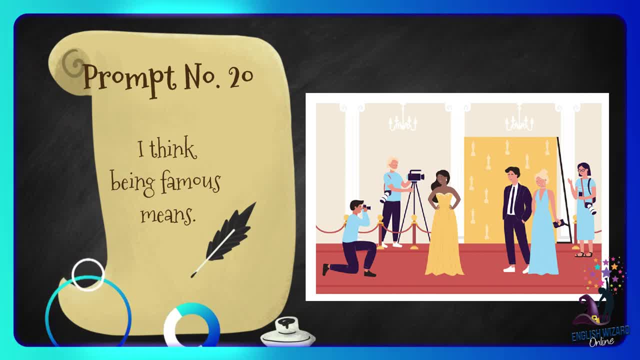 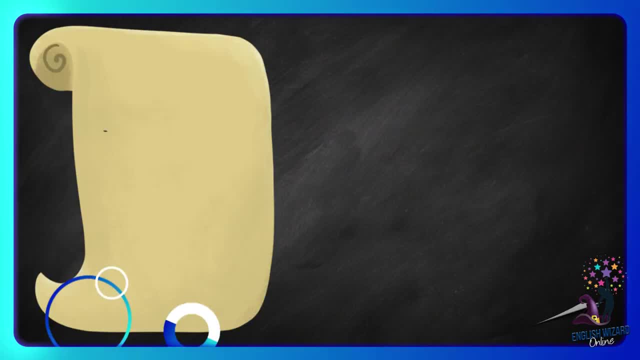 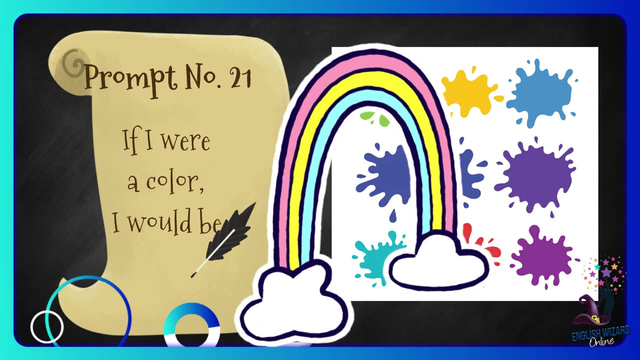 Other people may become famous for things they do, both good and bad. What do you think it means to be famous? Write about it Writing. Prompt Number 21: If I were a color, I would be. Color is more than a visual experience. 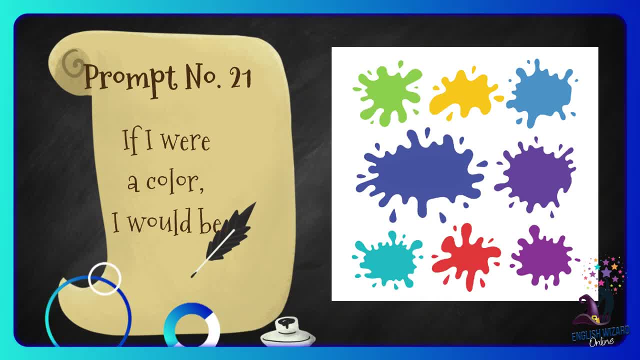 It is also a psychological one that can radically affect mood and emotion. Warm colors like red, yellow and orange can produce feelings of warmth or aggressiveness, while cool colors like green and blue can be calming or depressing. If you were a color, what would you be? 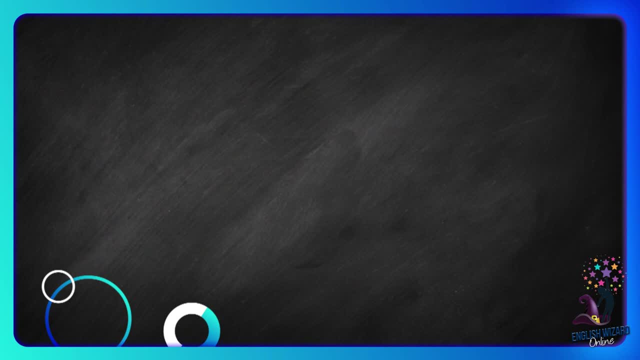 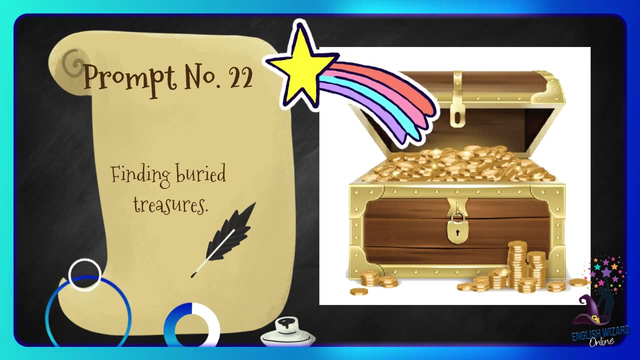 Write about it. Writing Prompt Number 22: Finding Buried Treasures. Buried treasure is a literary trope commonly associated with depictions of pirates, criminals and Old West outlaws. While some buried treasures have been found, there's still plenty out there just waiting to be discovered. 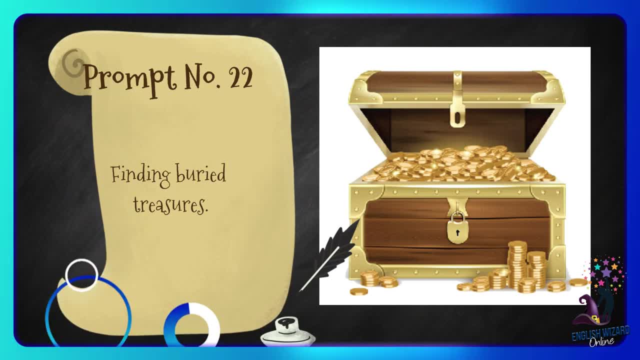 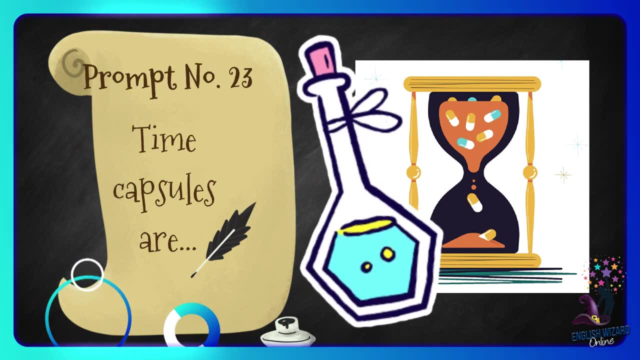 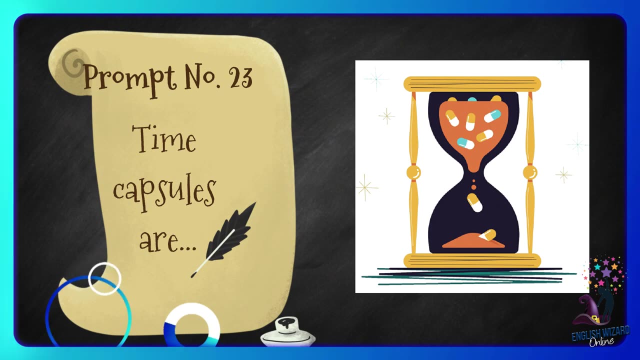 Imagine that you've found buried treasures. write about it. Writing. Prompt Number 23: Time Capsules Are. A time capsule is a historic cache of goods or information, usually intended as a deliberate method of communication with future people and to help future archaeologists, anthropologists or historians. 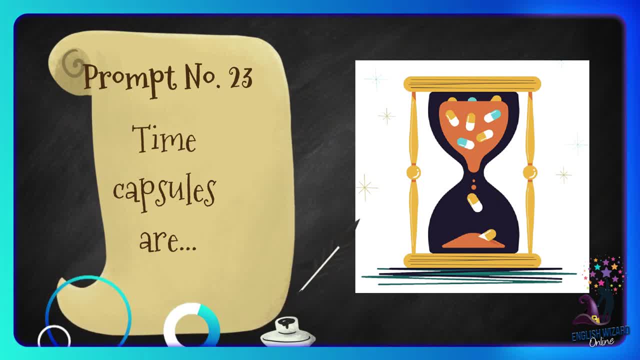 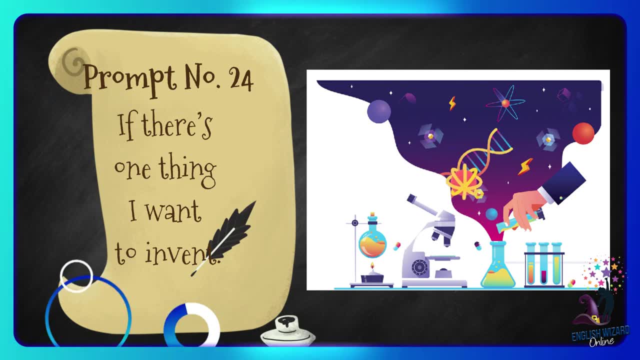 What do you think about time capsules? Write about it Writing. Prompt Number 24. If there's one thing I want to invent, an invention is a unique or novel device, method, composition or process. If there's one thing you want to invent, what would it be and why? 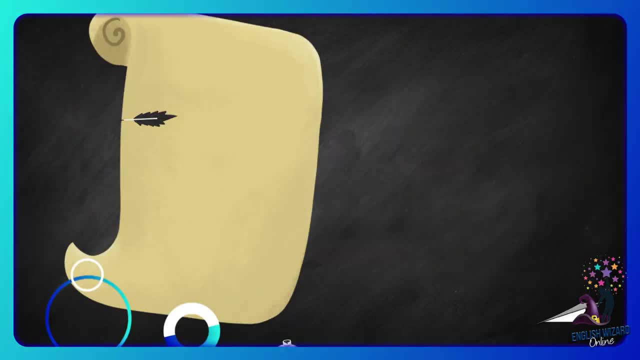 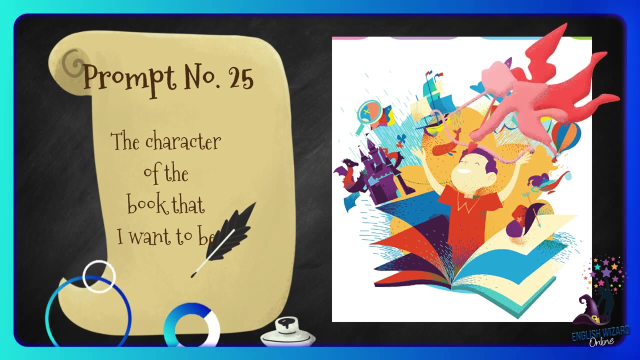 Write about it. Writing Prompt Number 25: The Character of the Book That I Want to Be. In fiction, a character, or sometimes known as a fictional character, is a person or other being in a narrative such as a novel, play, television series, film or video game. 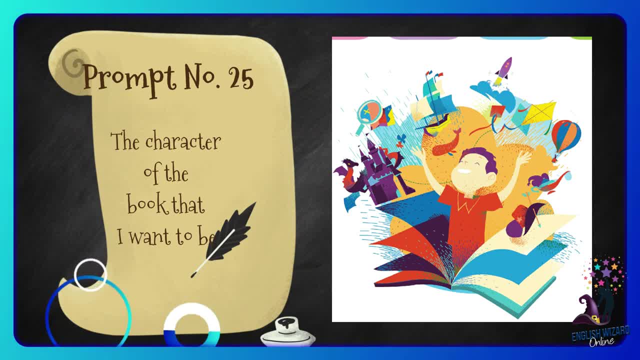 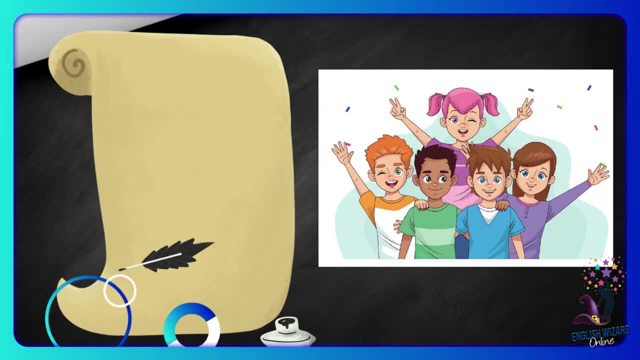 You probably read many stories with interesting characters. Write about the character you want to be. Write about the character of the book that you want to be Writing. Prompt Number 26. I think I don't think we should fight for a friend. There are some things that are worth fighting for. 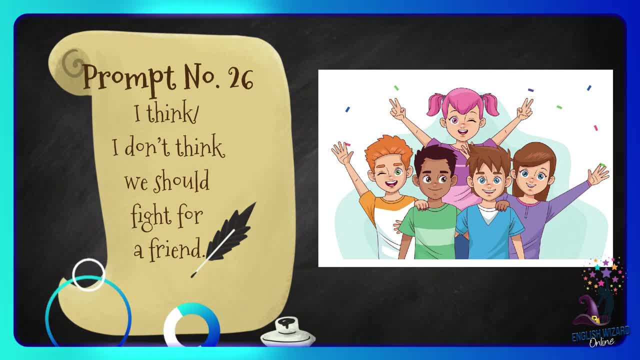 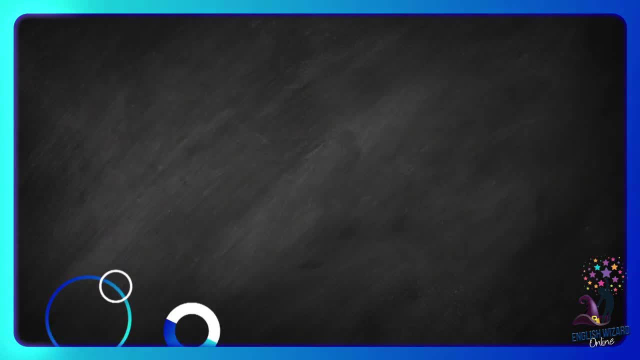 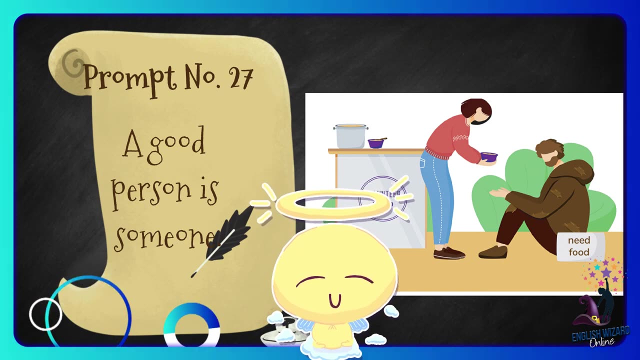 We should fight for our families, we should fight for our future and maybe fight for a friend. What do you think about fighting for a friend? Write about it. Writing Prompt Number 27. A good person is someone. The term good has relative meanings depending on the person who is defining it. 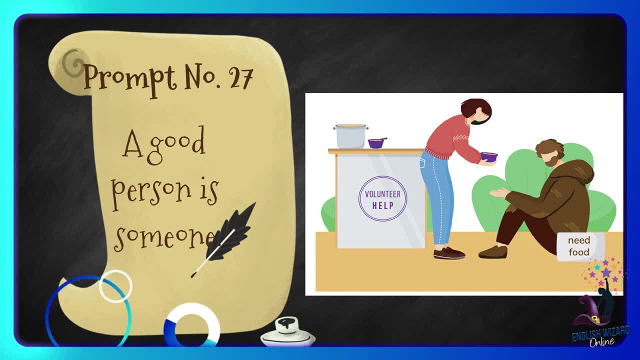 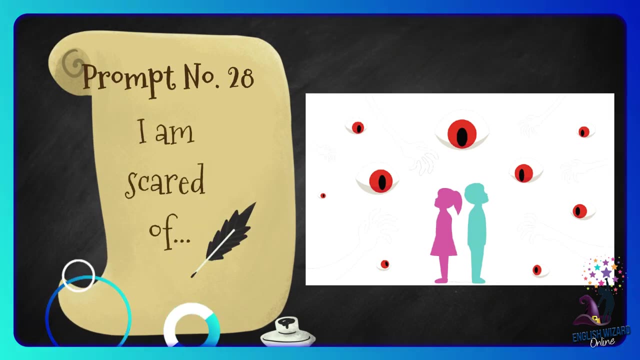 Several qualities can be used to define what constitutes a good person. However, there are certain basic qualities that are used to define a good person. Write about who you think is a good person. Writing Prompt Number 28. I am scared of People, feel scared once in a while with different things. 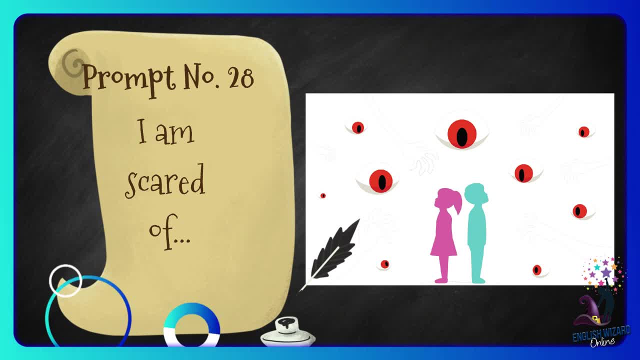 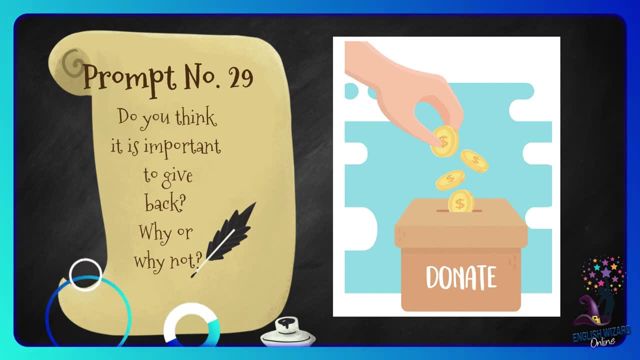 What are you scared of? Write about it. Writing Prompt Number 29. Do you think it is important to give back? Why or why not? Sometimes, giving back to the community is as simple as giving time, money and old belongings. Do you think it is important to give back? 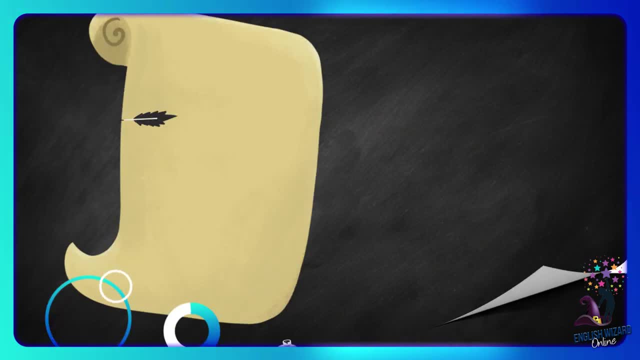 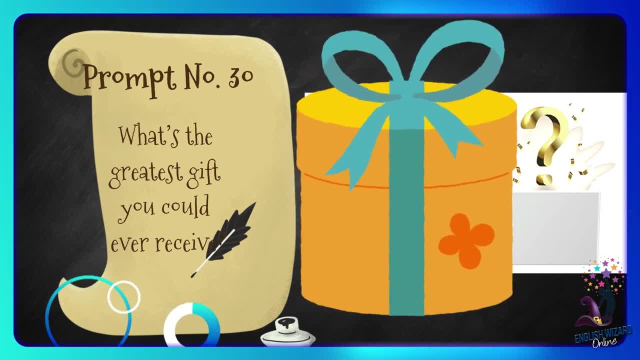 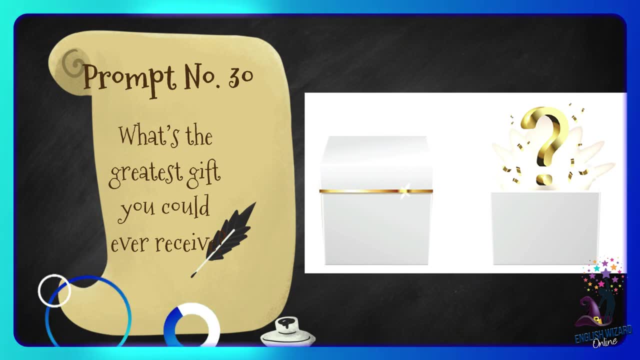 A gift or a present is an item given to someone without the expectation of payment or anything in return. An item is not a gift if that item is already owned by the one to whom it is given. Although gift-giving might involve an expectation of reciprocity, a gift is meant to be free. 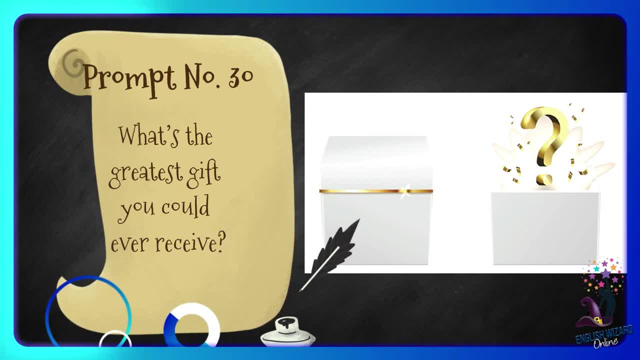 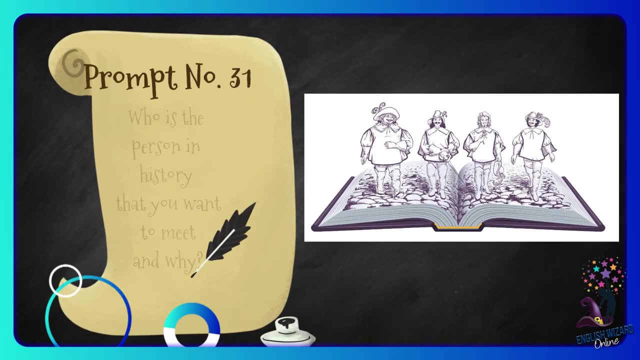 What's the greatest gift you could ever receive? Write about it. Writing Prompt Number 31: Who is the person in history that you want to meet and why? History helps us develop our knowledge of history. It helps us develop a better understanding of the world. 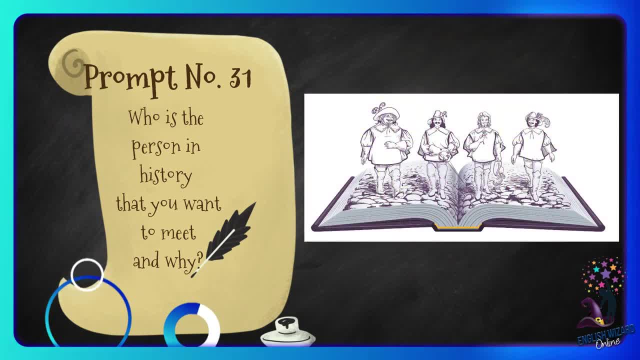 You can't build a framework on which to base your life without understanding how things work in the world. History paints us a detailed picture of how society, technology and government worked way back when, so that we can better understand how it works now. It also gives us a glimpse of different people who shaped course of history. 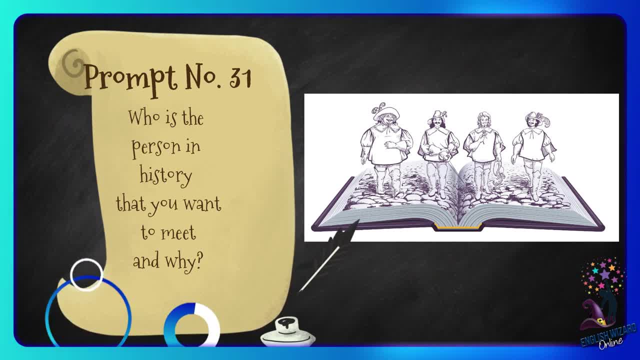 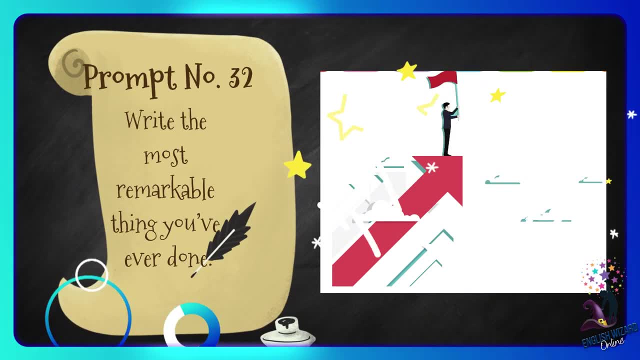 Who is the person in history that you want to meet and why? Writing Prompt Number 32, Write the most remarkable thing you've ever done. Something remarkable is unusual, exceptional, interesting or excellent. Remarkable things. get your attention. Write about the most remarkable thing you've ever done. 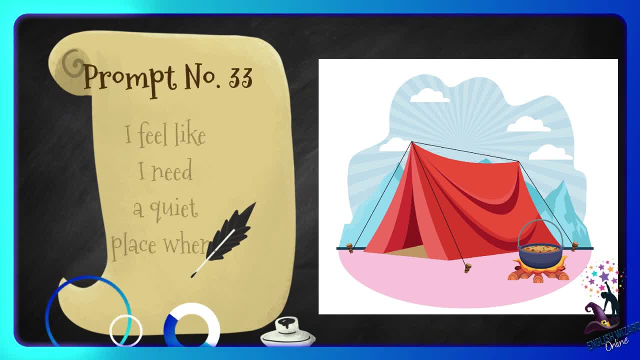 Writing Prompt Number 33, I feel like I need a quiet place. when A quiet place is characterized by an absence of turbulent motion or disturbance, It is peaceful, calm or tranquil. It is characterized by an absence, or near absence, of noise. When do you feel like you need a quiet place? 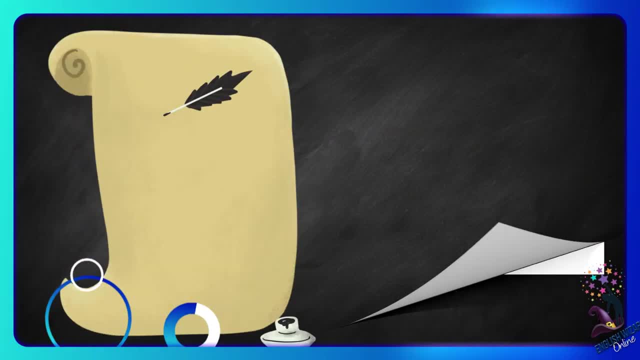 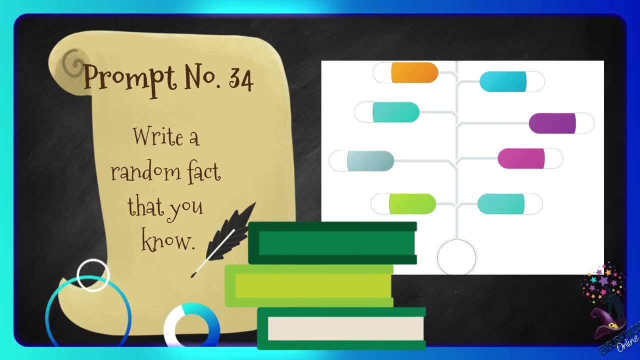 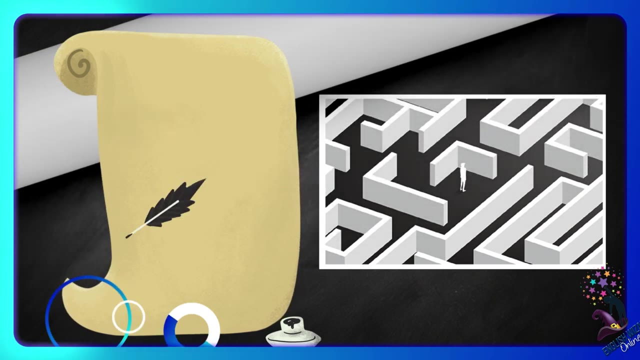 Write about it. Writing Prompt Number 34. Write a random fact that you know. Facts are pieces of information that can be discovered. Write about a random fact that you know. Writing Prompt Number 35. Getting lost in a maze would make me feel. 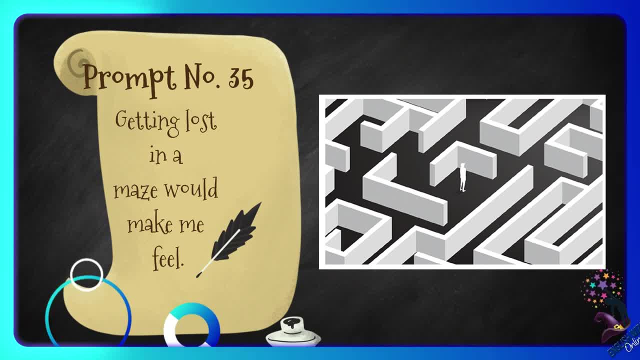 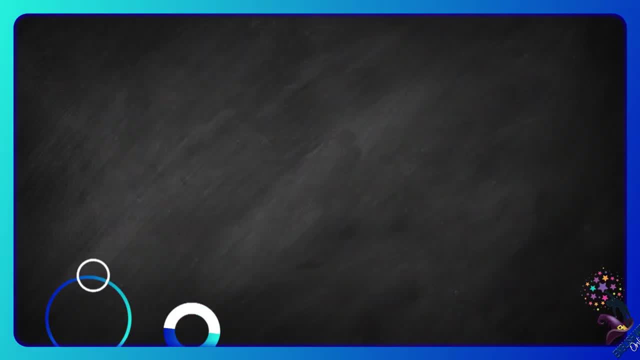 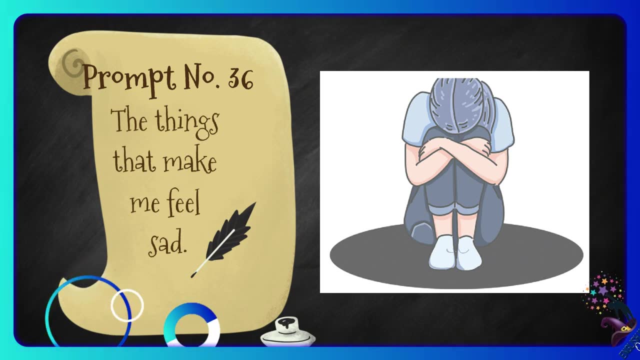 In mazes with miles of paths, it's no surprise that people get lost. How would it make you feel? Write about it. Writing Prompt Number 36: The things that make me feel sad. Sadness is an emotional pain associated with or characterized by. 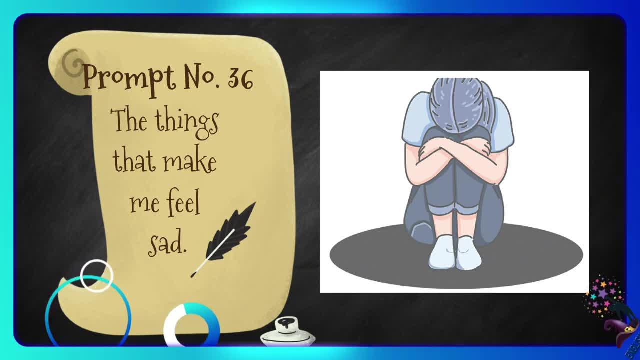 feelings of disadvantage, loss, despair, grief, helplessness, disappointment and sorrow. An individual experiencing sadness may become quiet or lethargic and withdraw themselves from others. What are the things that make you feel sad? Write about it. 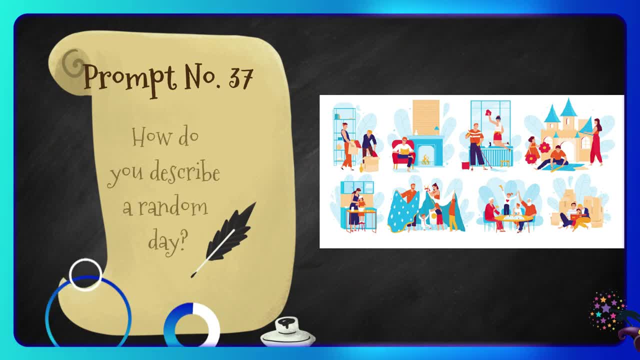 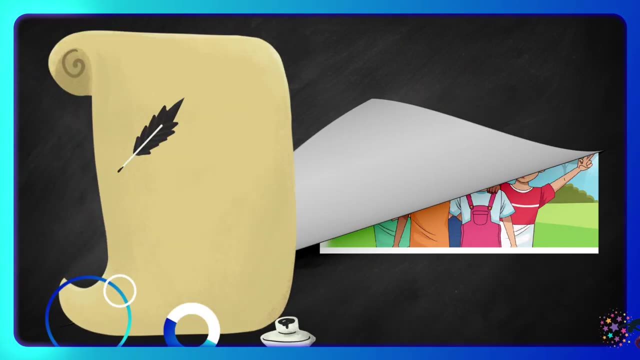 Writing Prompt Number 37. How do you describe a random day? At random means, by chance or without any organization or plan, unexpected and surprising. Describe a random day. Writing Prompt Number 38. Writing Prompt Number 38. What do you like the most about yourself? 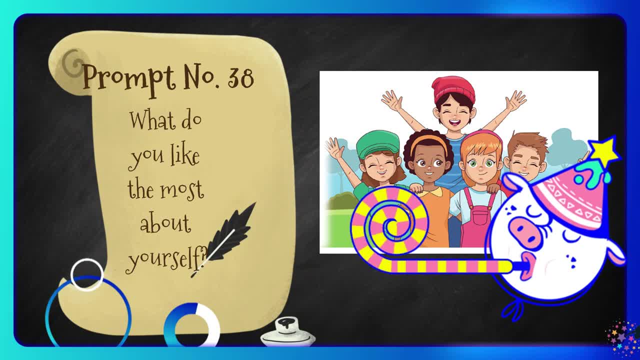 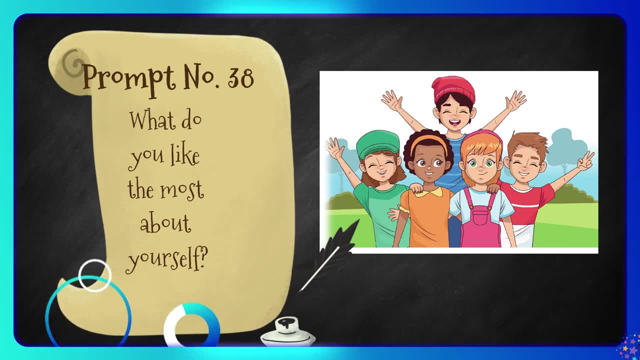 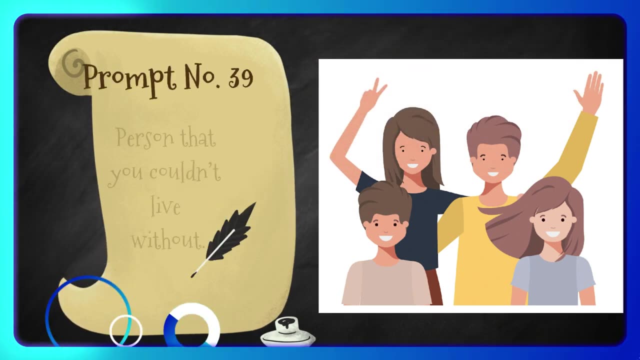 What do you like the most about yourself? Coming up with things you genuinely love about yourself is a valuable exercise. Write about something that you like the most about yourself. Writing Prompt Number 39 Person that you couldn't live without. People are meant to spend time with other people.